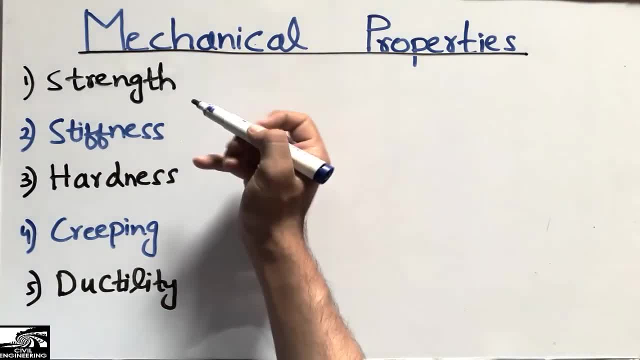 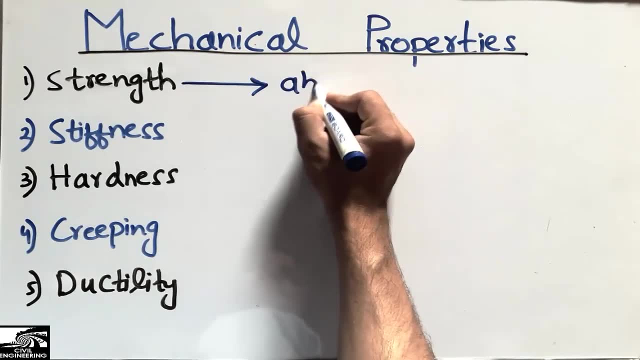 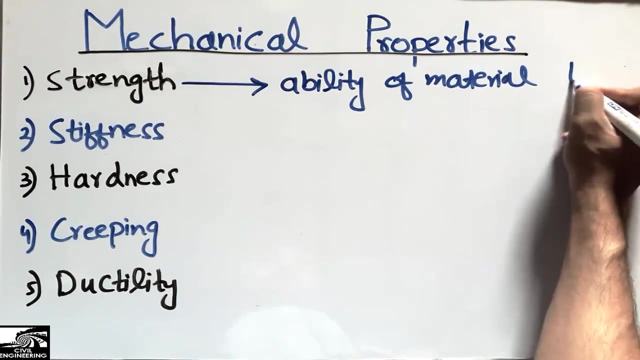 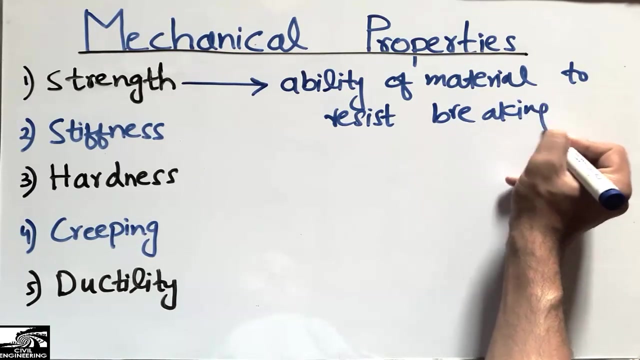 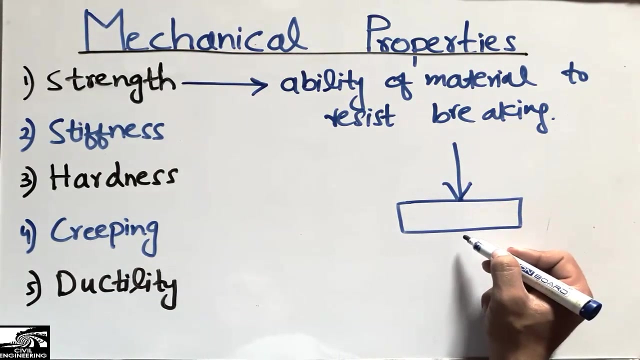 So the first property of the material- mechanical property we can say- of the material- is the strength. So strength is the ability of the material to resist what, To resist breaking, For example, consider this is in a material block and the load acts on this block. So what happens? 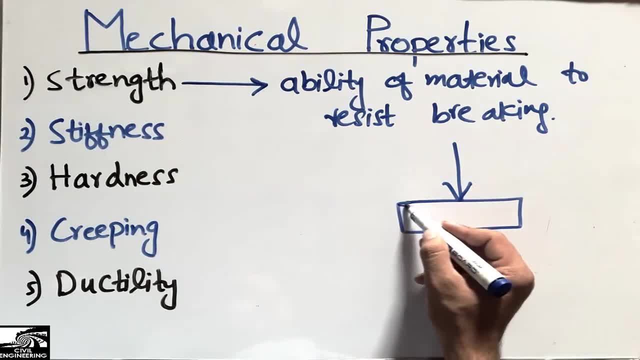 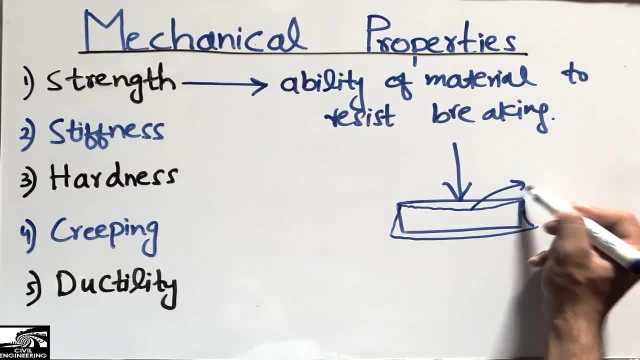 It will take the load. this block will take the load, will take the load until it takes the load Fractures and it breaks. So we call is that this material is now breaks. So the load resisting capability of this material until it breaks we call is the strength of material. 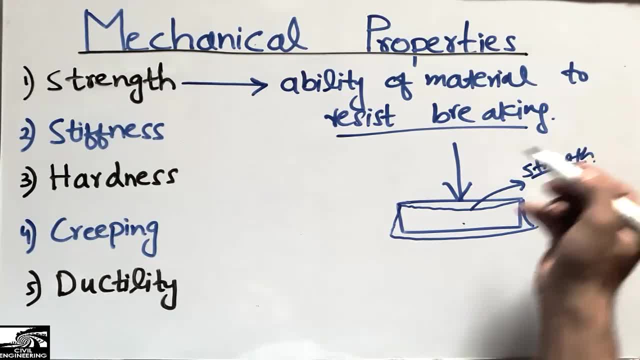 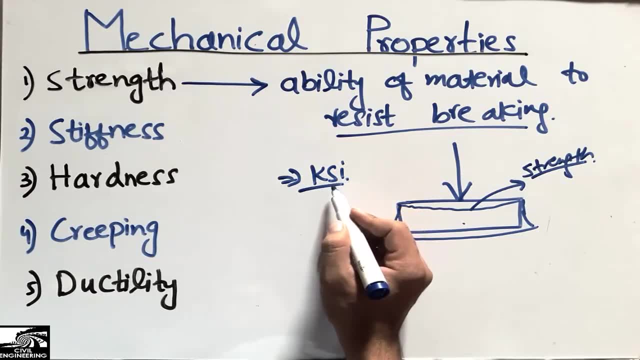 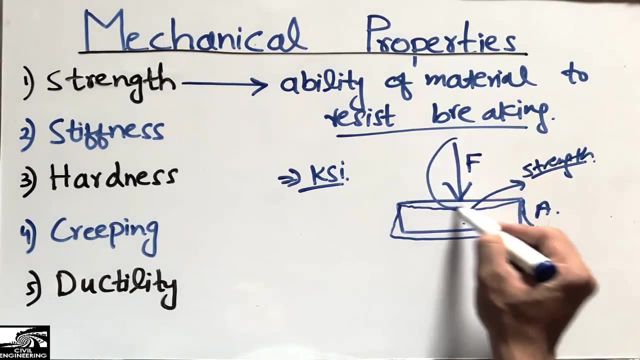 This is the strength of material and the strength is usually measured in the KSI K per pound square inches, And the unit of it means the force per unit area. It is the force in this area of the material. So the load acting on this material up to the up to when it breaks we call, is the strength of material. 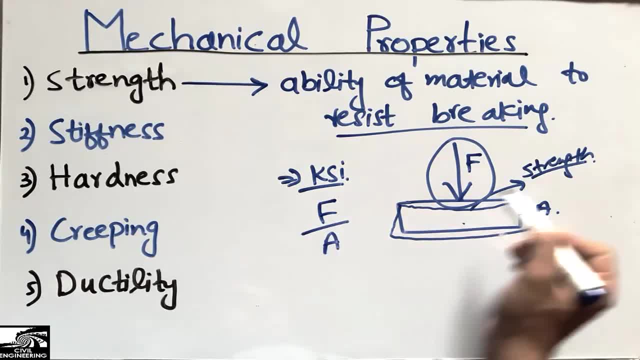 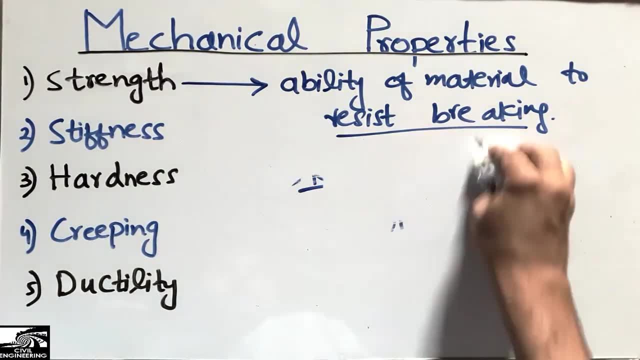 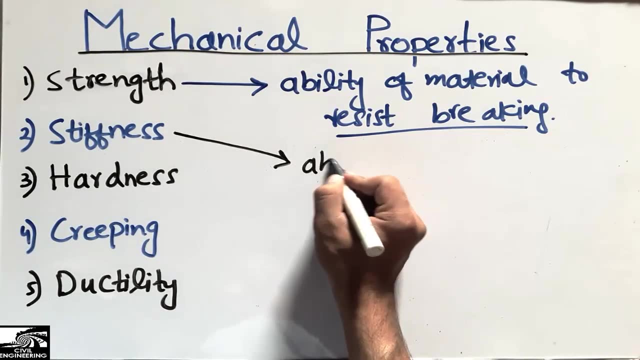 So the force per unit area we call is the strength of material. The second property of the material is the is the stiffness of the material. It is little bit different from that of the strength of the material. Strength stiffness is the ability of a material. 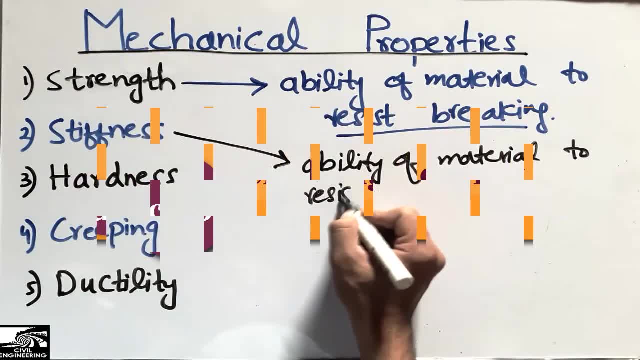 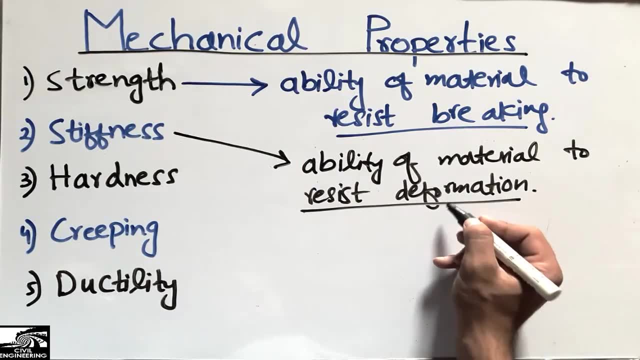 the ability of a material to resist deformation. to resist deformation, It is not the strength, It is not the breaking, It is related to the deformation of a material. For example, consider the same block and the load acts on this block. So the material will now deform upon loading, So it will follow this path. 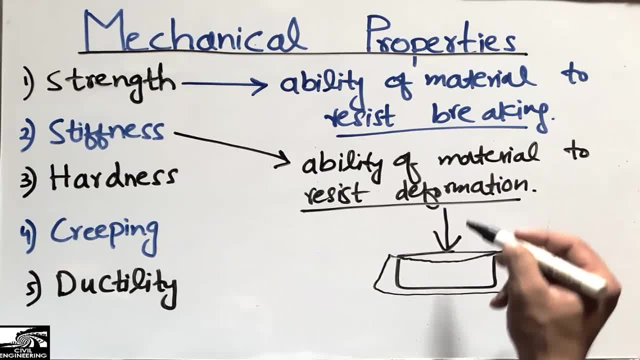 So we call is the when this material resists the deformation, the load acts and it resists this deformation Not to occur this deformation and to not to occur this deformation. So this resistance to deformation we call is the stiffness of material. The more the resistance to deformation, the more will be the stiff material. 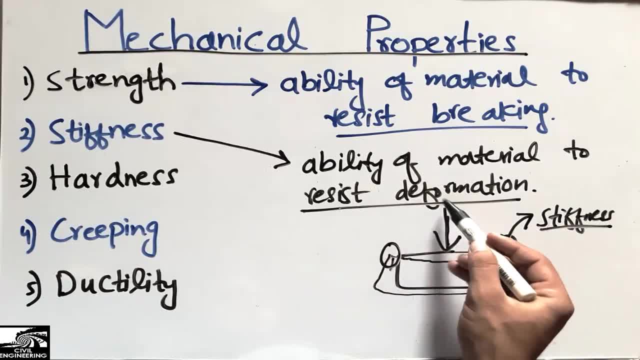 The less will be the flexible material And the less the deformation of a material is means the more stiff is a material And the more deformation, the less stiff is a material. So everything I have explained was done by� Yes, sir. 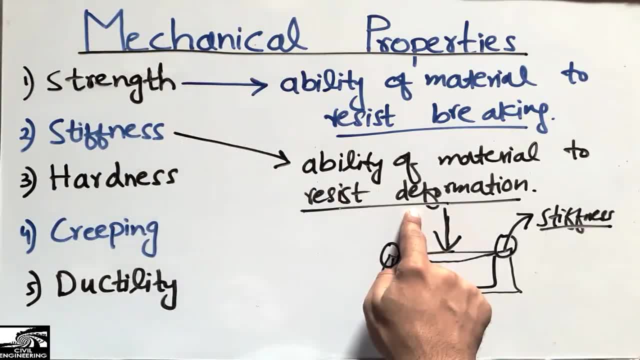 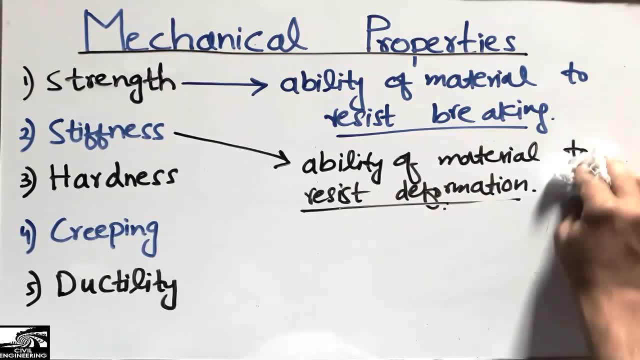 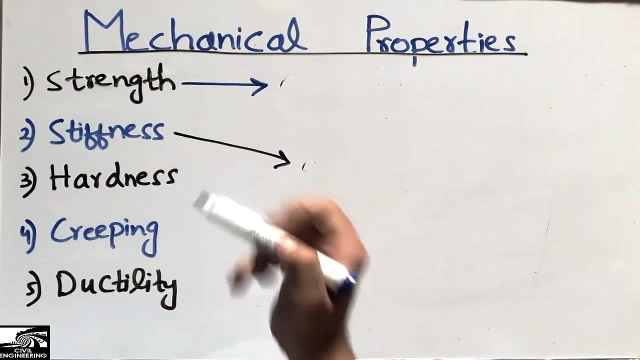 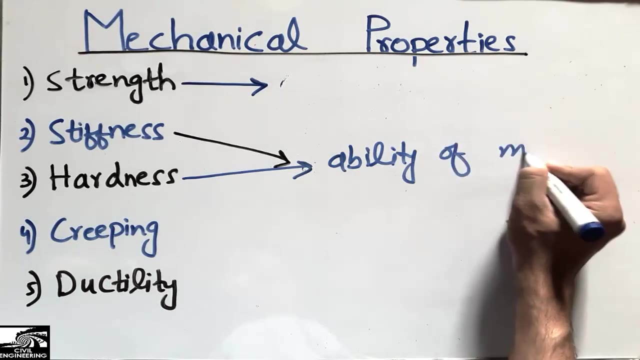 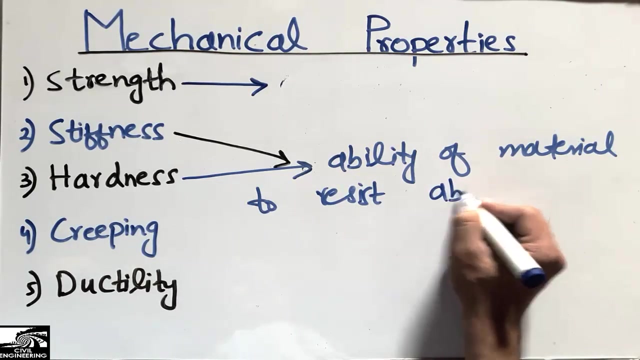 sir, is totally related to the deformation of a material. it is the resistance to the deformation. the third property of material we can- we can write it here- is the hardness of the material. hardness is the ability of material, ability of material to resist, to resist creaching are, to resist abrasion. we call this. 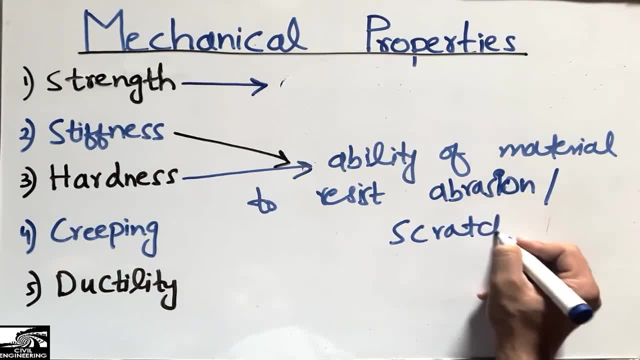 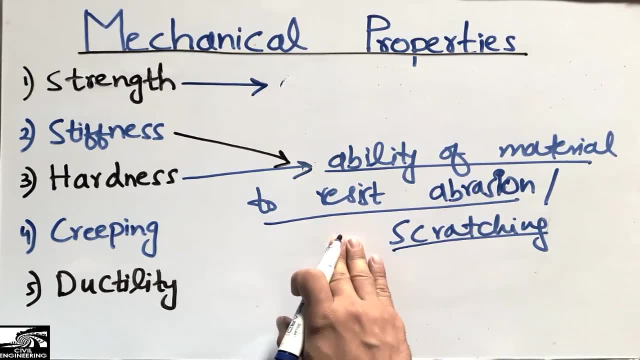 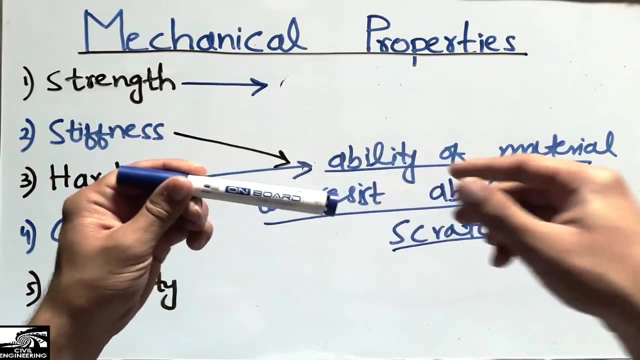 property straight, ensure the impression we called this type of property, of the material we call easy, hardness it, how much it like. for example, consider any like this is a material and I'm going to slide over this material and how much this material give me aließha. 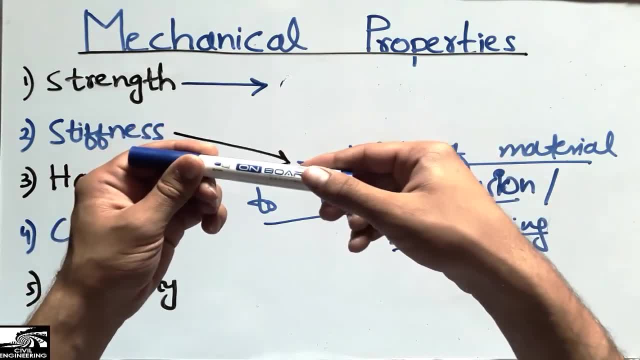 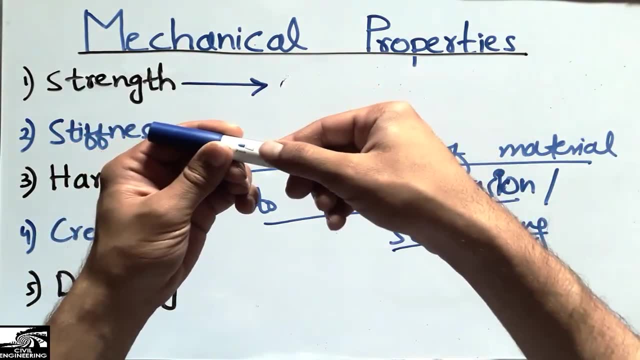 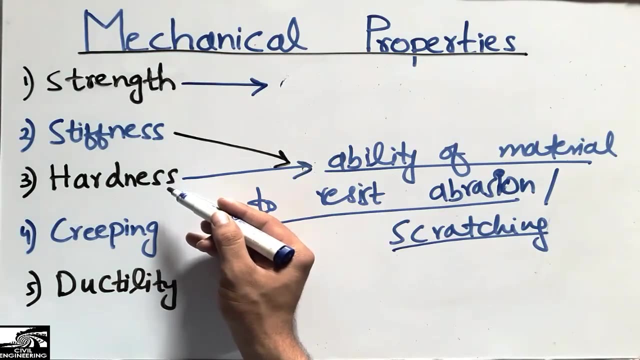 the screeching phenomena or the screeching ability. so this we can say is a hard material. if the- if my hand goes on slightly- or this material, we cannot say there is a hard material, because this is a soft material. but more give it abrasion we call easy, the more is the hard material. so totally. 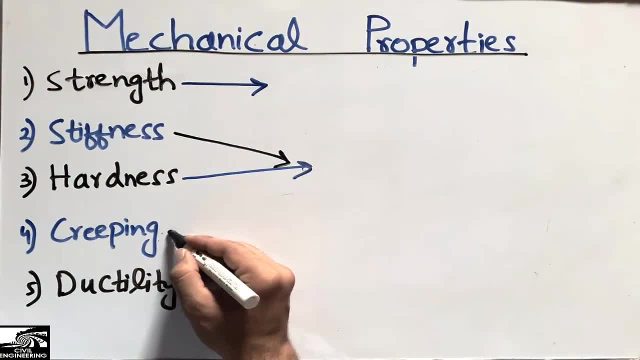 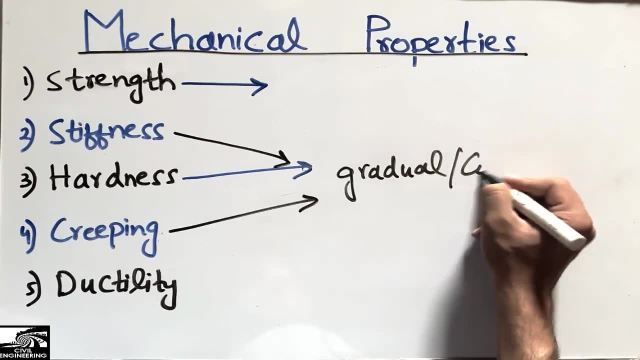 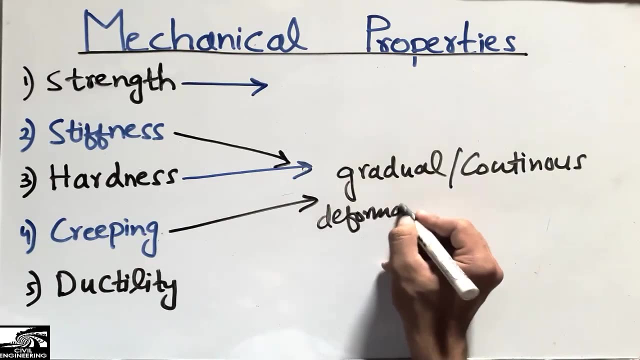 related to the abrasion of the material. now, coming to the fourth property of the material: creeping. creeping is a gradual as a gradual, or the continuous or the continuous deformation of a material. continuous or gradual deformation, deformation of a material under under constant, under constant stress. it is the uh, it is the constant, it is the continuous. 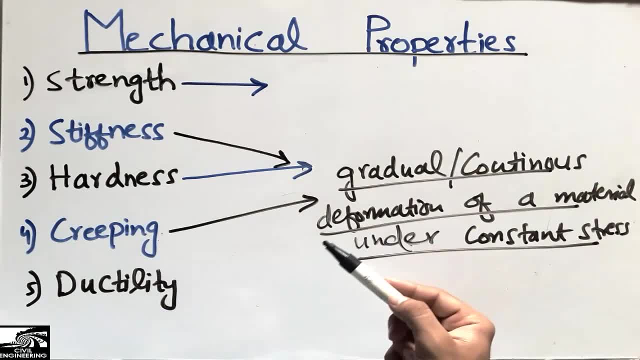 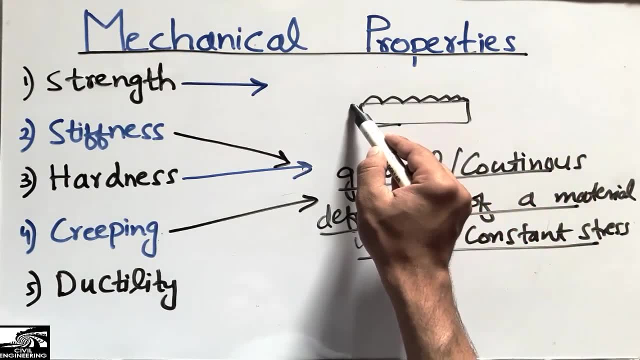 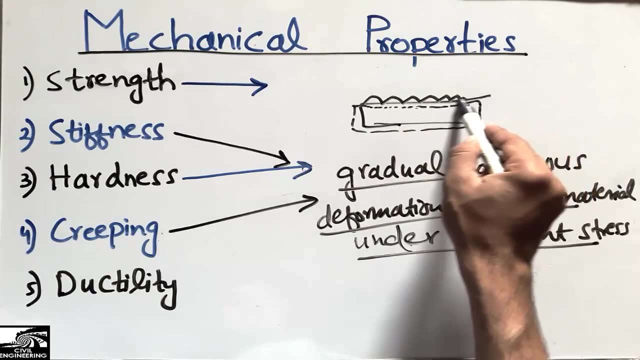 it means it the creeping, the behavior of the material. for example, this is in a concrete block and this load x on this concrete block. so it will deform with the time with. after 10 or 20 years it will deform like this and this deformation continues with the time, upon the constant. 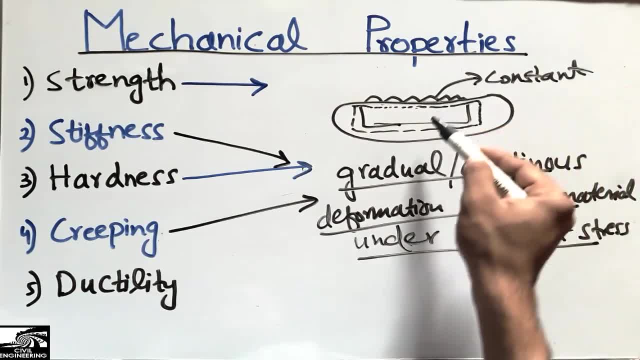 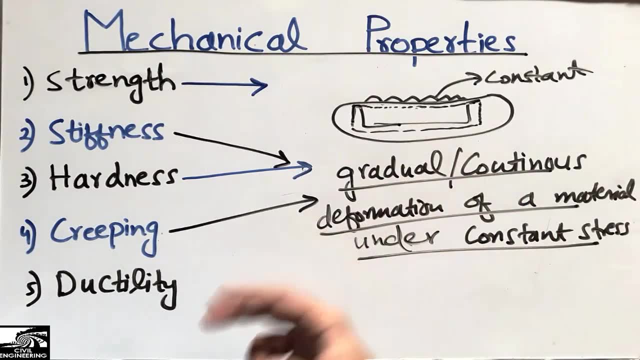 stress on this material. so this constant deformation of this material with time we call the creep of the material. so this is the property of concrete, usually that it goes uh, the deforming, the wave time, so we call, is the creeping of the material. now coming to the last property of the 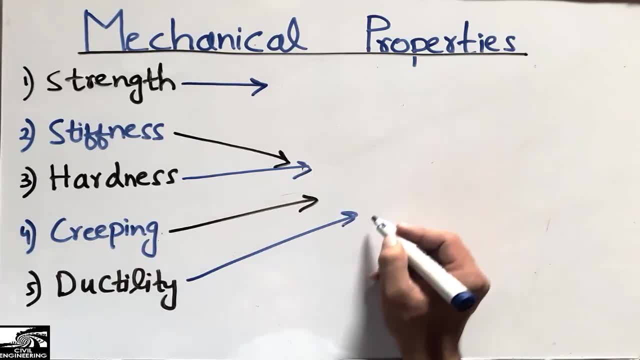 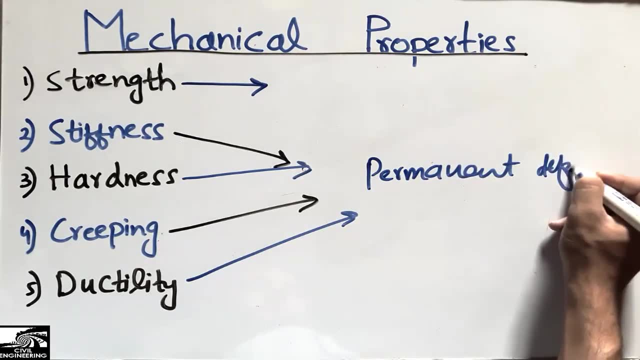 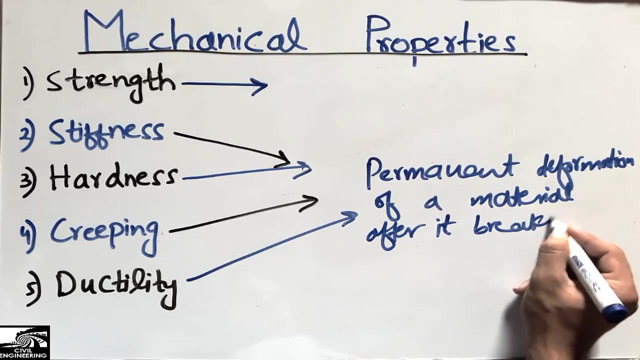 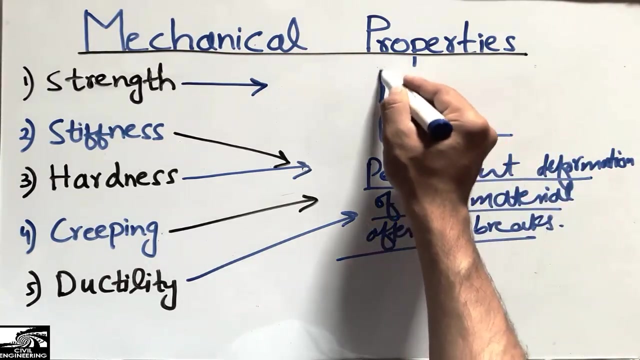 material. it is the ductility of a material, ductility and ductility as the permanent deformation of a material. permanent, permanent deformation, deformation of a material after it breaks, it is the permanent. for example, consider this the stress strain graph: this is here the stress, here is the strain. so when the load x in the body, it will follow. 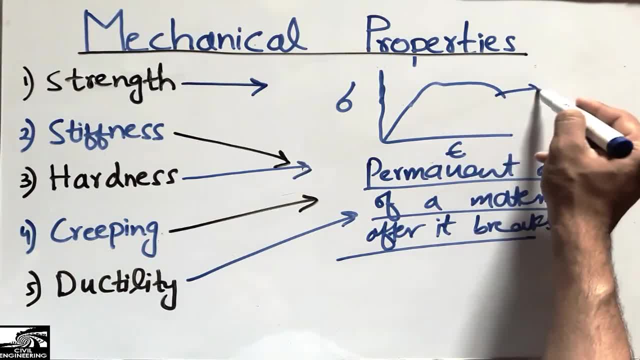 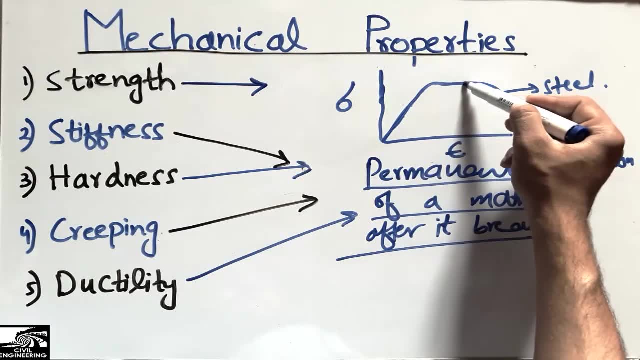 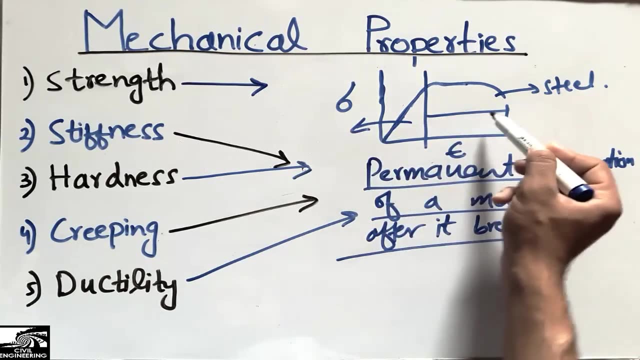 this path. for example, this is the steel graph, so it will follow this path. so we have to achieve the variation 200 by the plastic deformation after it breaks the material with a знач красim passing here. it follows this particular layer and follows this path in the load. 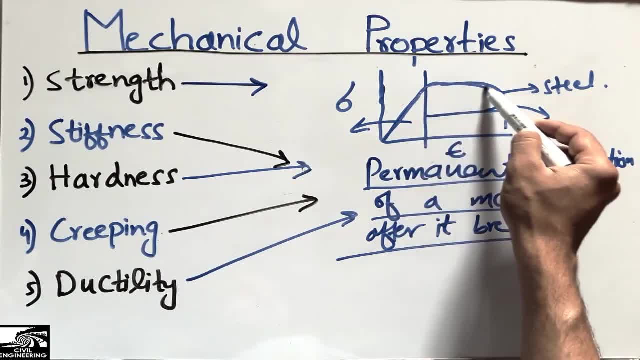 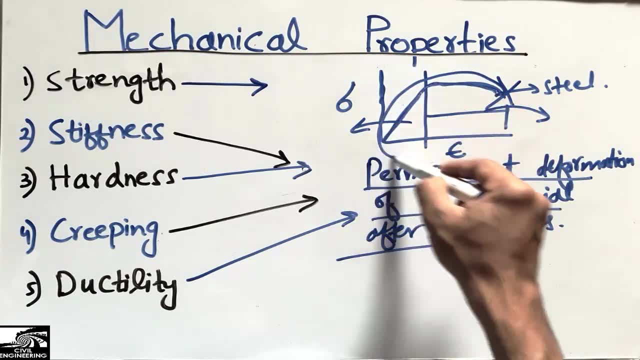 it take, it takes the load and after this it will start the plastic deformation here from this point onwards it is the elastic deformation. at this point it is the plastic deformation here at this stage. so the permanent deformation after this it means the permanent deformation of a material after. 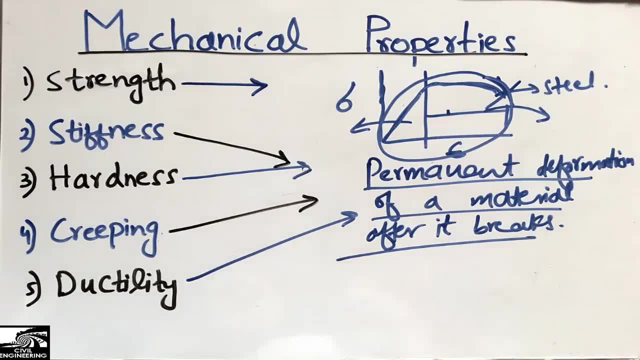 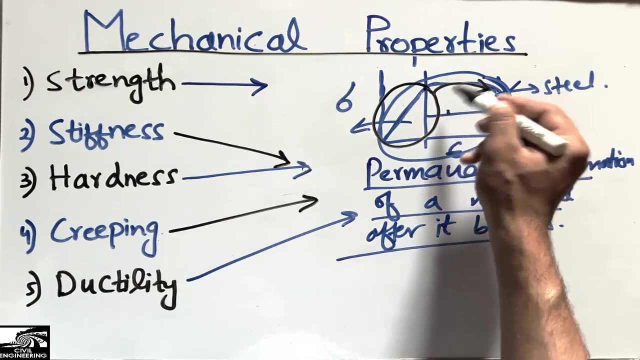 when it bricks at this point, the more permanent deformation here occur in the material and the more ductile will be the material. and inverse of this material is the brittle material. the brittle material actually fails at this point. it don't goes after the plastic deformation, so we call it the brittle material. 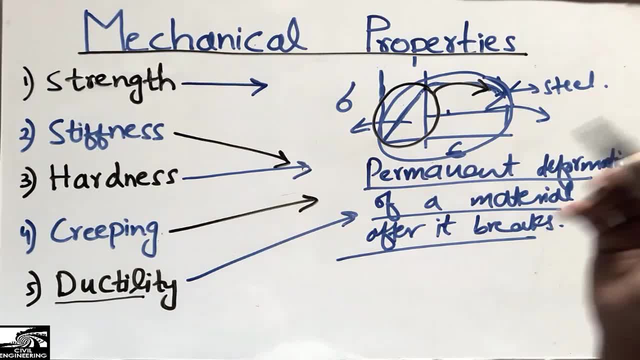 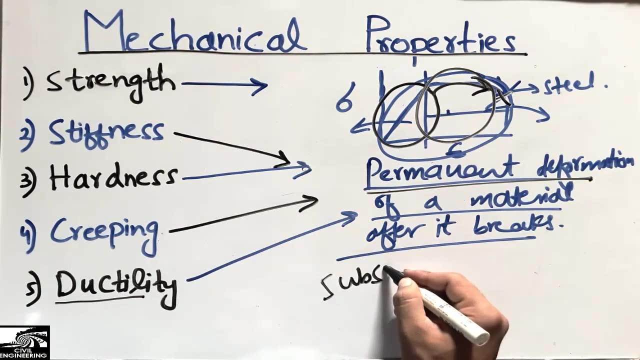 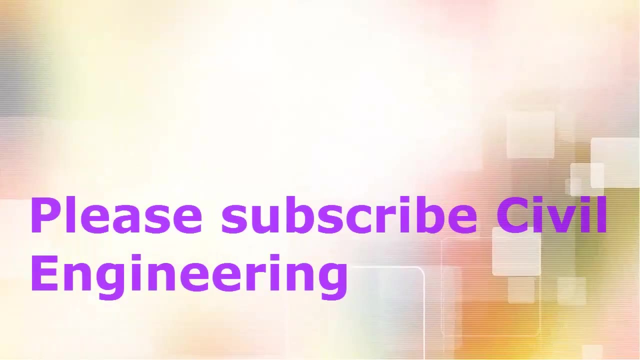 while ductility is that property which it is the permanent deformation of in a material and after which it breaks down. we call it the ductility of the material. this was all about the mechanical properties, or you can watch more videos and subscribe our channel for daily seo engineering videos. thank you for watching our video.